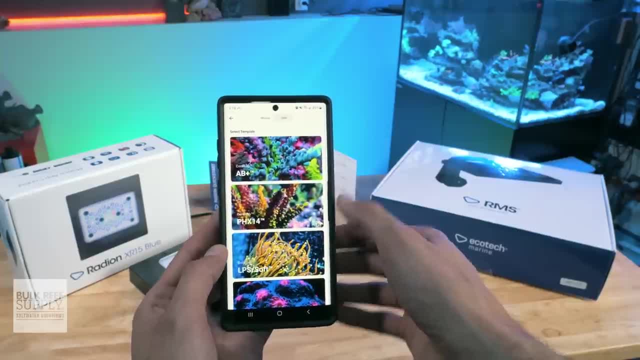 sliders Instead, preview the various presets that your LED fixtures will have. So if you're looking for a light that fits your goals, pick the one that the LED light provides you with, and choose the one that looks best to your eye. Or if they have descriptions as well, you can choose the 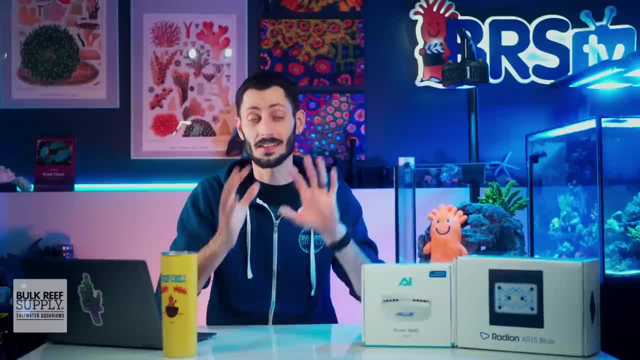 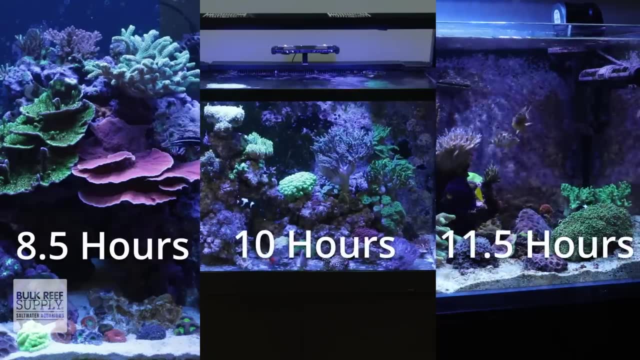 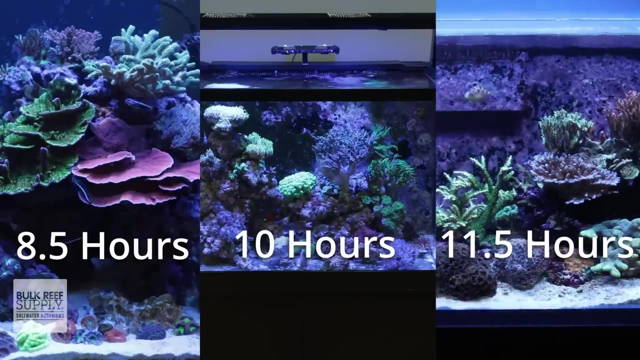 one that best matches your reefing goals. Once you've got the spectrum down, that's where the 1-8-1 ratio comes in. There's no 100% right answer when it comes to how long the light should be on, for Some of us run shorter light schedules than others. Some of us like long ramp times, while 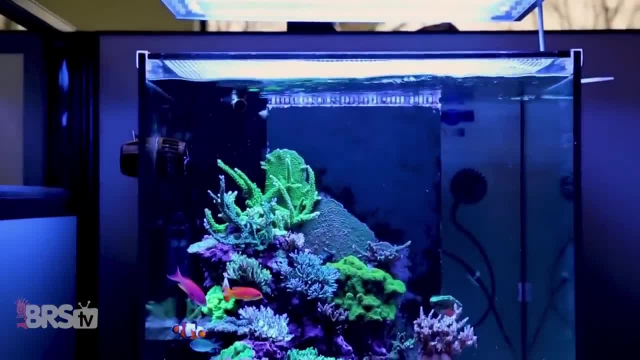 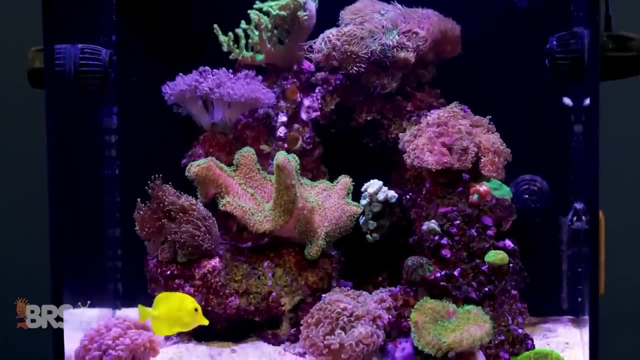 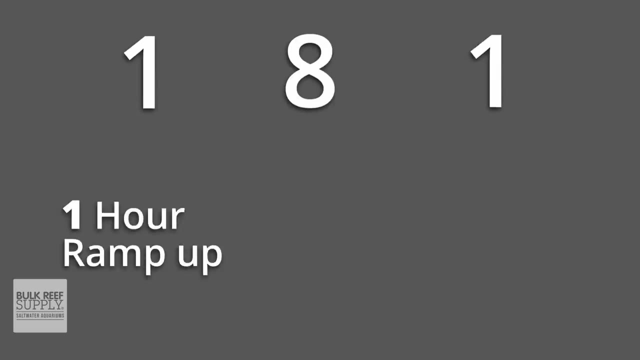 others prefer shorter ramp times. Those preferences come from a lot of experience with our individual tanks. For those of us who don't yet have that experience, the 1-8-1 ratio is a perfect starting point and you may never want or need to change it. 1-8-1 means one hour ramp up, eight hours full. 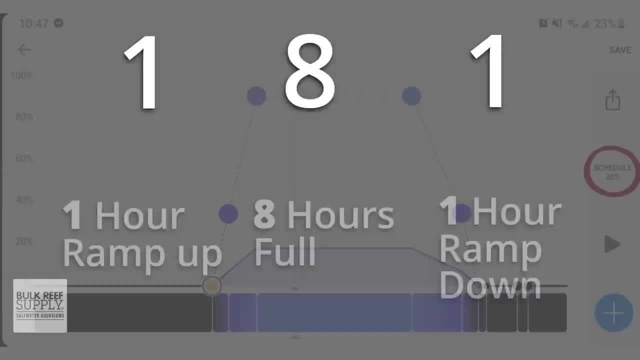 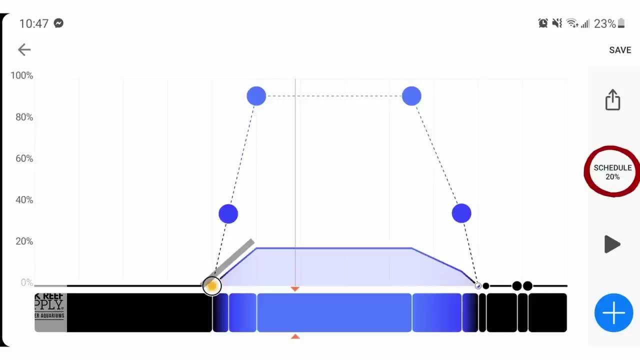 intensity and one hour ramp down. What this looks like for your light schedule is: whatever time the light comes on, it takes one hour to go from 0% to the maximum intensity, then stays at that maximum intensity for eight hours, and then takes one hour to go from that maximum intensity to the maximum. 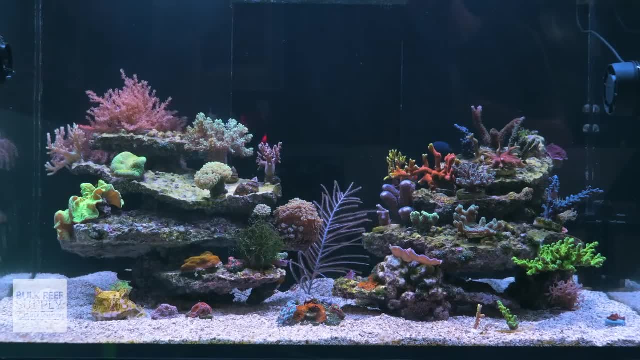 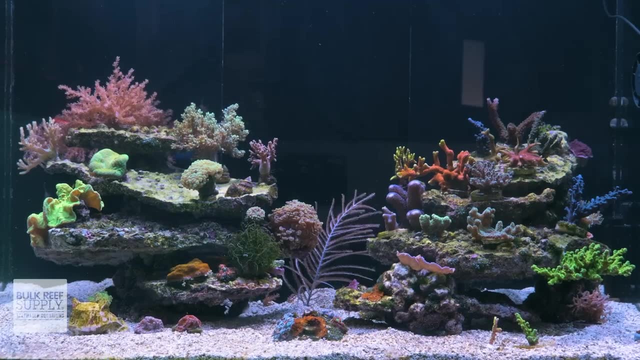 intensity back down to 0%. This gives you a 10 hour light cycle, which is right in the middle of the typical range of eight to 12 hours, and a successful schedule that many reefers, myself included, use The last thing that you will absolutely want to do when setting up your 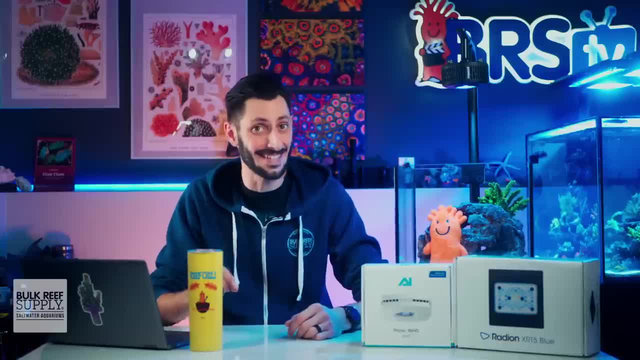 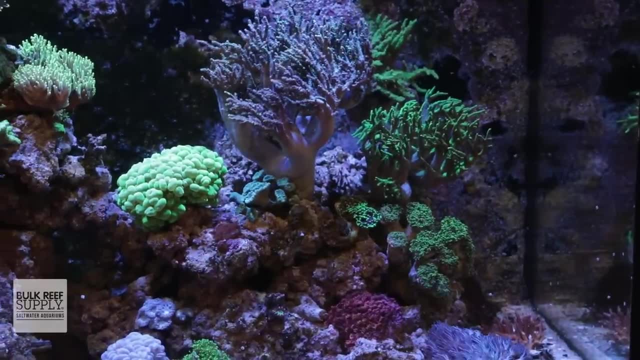 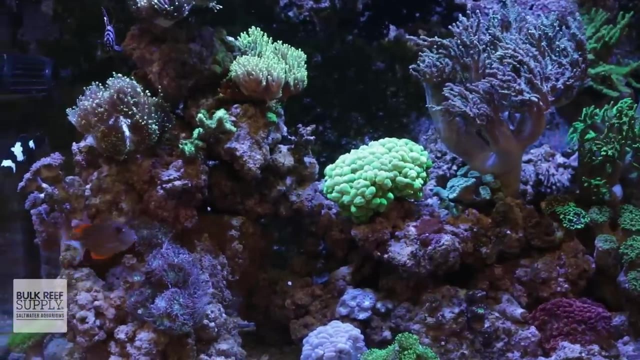 light schedule is: pick the best maximum intensity for your particular types of corals. To give you an idea of why this is so important, if you were to put softies or LPS corals under a light that is much too bright, they usually respond by bleaching, which will often lead to coral loss. 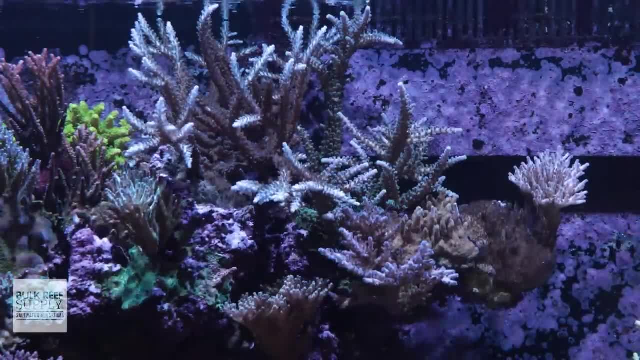 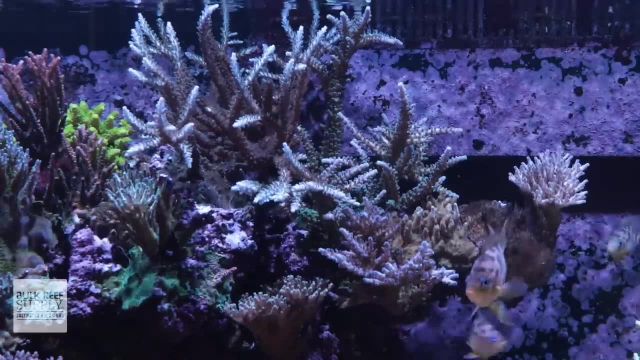 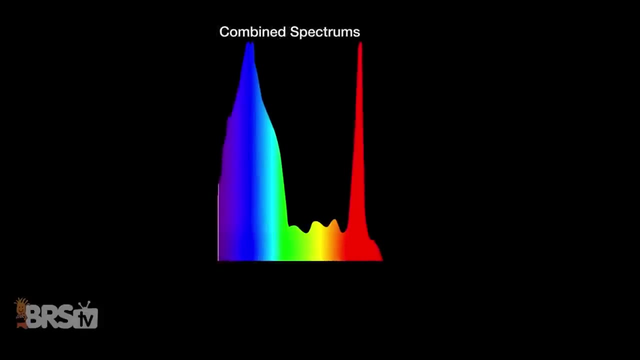 If you put higher light corals like SPS under a light that isn't bright enough, they can brown out, lose color, stop growing, and if the light is much too dim they too can perish Reef. lighting intensity or brightness is measured in PAR. PAR basically measures how much usable light is. 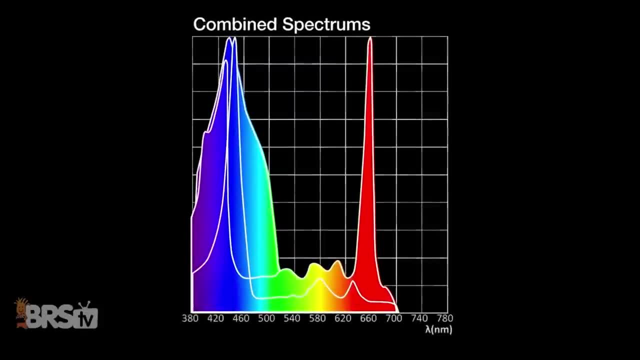 available for the corals to photosynthesize from a particular light source. A PAR meter is the tool that we use to measure the amount of light. if there's light in the corals that you put on a surface or if there's light that is on the surface, it does measure that If there's light on the surface.